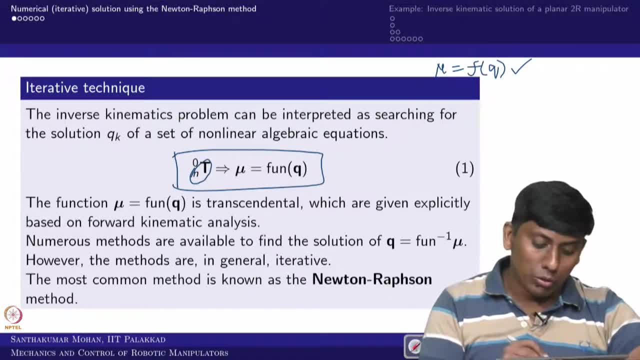 can say transformation matrix of nth with respect to 0, you can actually like, found, like, finally, what is your mu? So mu is actually like nothing, but sorry. end of vector positions. ok, So then you have actually like end of vector orientations. So this is what mu. 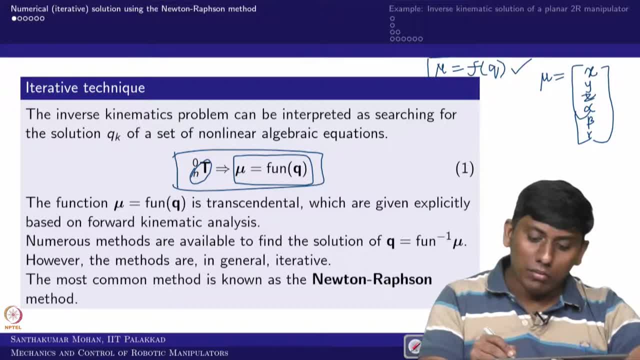 but we can actually like a generalize and all. So now, if you have this function, can I use any iterative method where I can find? if I give mu, can I find q? So that is the question. So if I have this big question numerically, there are several way So that. 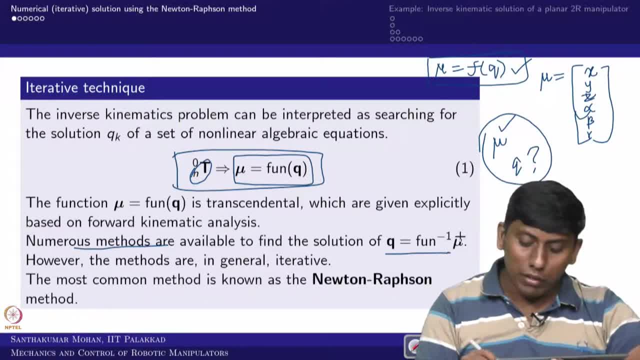 is what numerous methods are available to find this. q is actually like function of. you can say function inverse of mu, But we are actually like taking the iterative, because that is more general, and it it is actually like applicable to any kind of serial or parallel manipulator, In that one of the 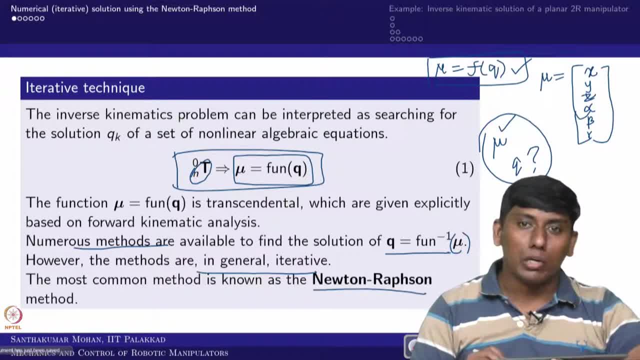 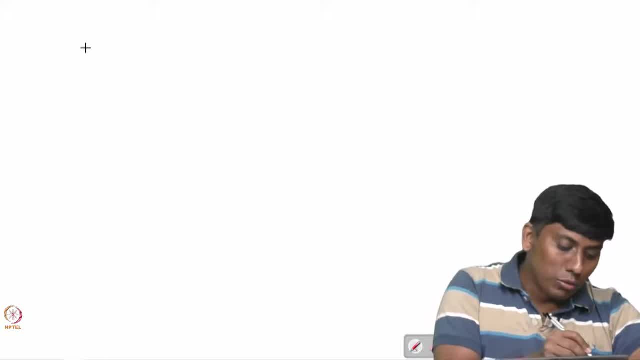 popular method we call Newton Raphson method, even some people shortly call Newton's method. So this is what we are actually like trying to see. So for seeing that I am actually like trying to show one thing. So this Newton Raphson method is actually like mainly come. 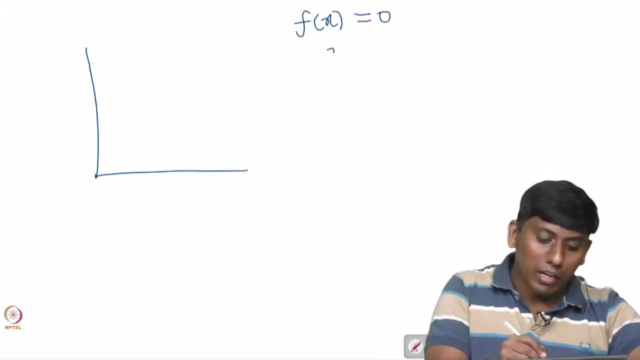 with this. So if function of x equal to 0, can I actually like find the solution x? So for that we are actually like taking a plot x versus you can say f of x. ok, So now I am actually like trying to show this So you can see like 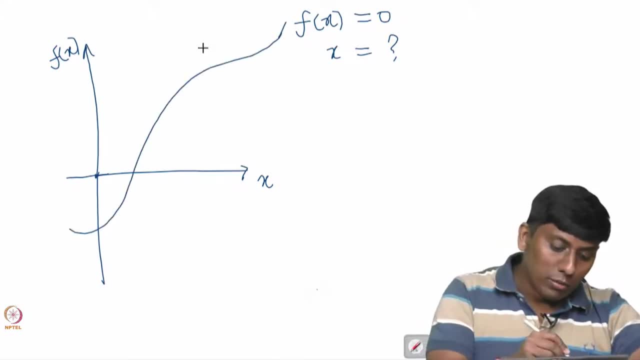 this is actually like somewhere like this: ok, So this is your function of x and this is actually like with respect to x. So now you can see like I am taking a random point, I will just complete this. So I am taking a random point, which I say, the initial guess. 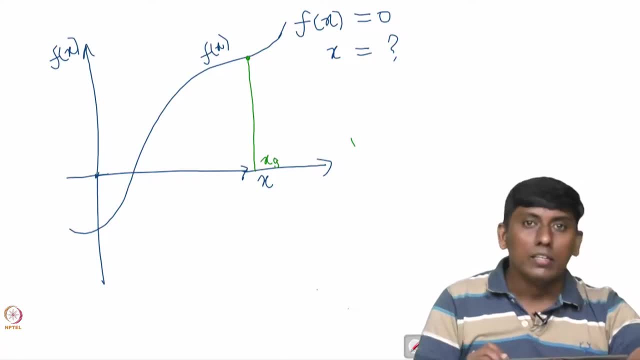 So this is actually like I call x, guess. ok. So now, so what I can do, I can actually like a make a slope, So I will just make it. this is little more ok, So something like this. So I am actually like a trying to plot, So I will, just because I did not properly. 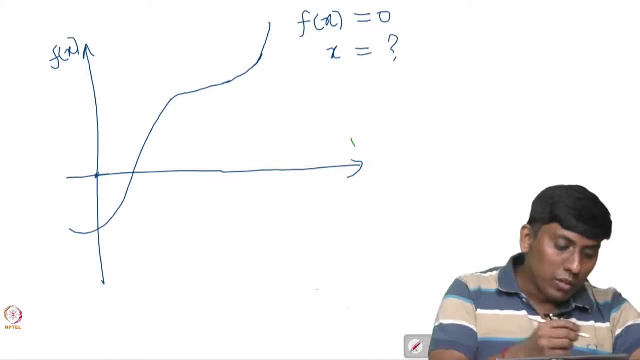 make it ok. So now I am taking a guess. So this is your function x, So x plus i will x, something like this: this is what my initial guess. ok, So, which I call x, g. ok, So now. 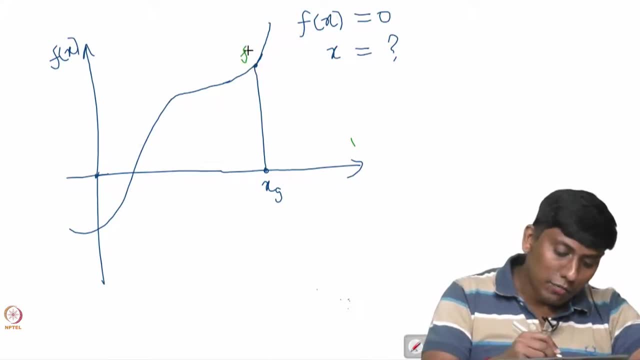 what we are actually like, seeing that the slope I can find and the function of x, g, I can find. the slope I can find. the slope is actually like coming like this: ok, So this is the f dash of x, g, So this, so now what you can see. this is actually like ending. 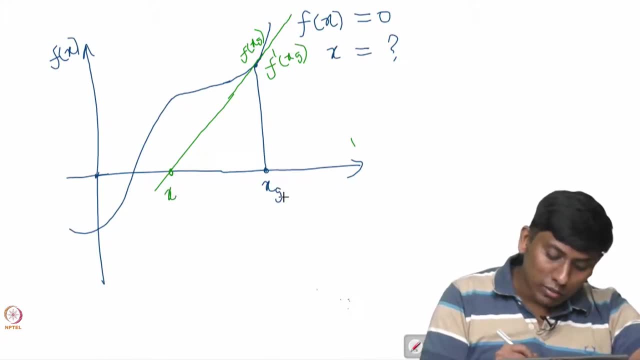 on the x somewhere. I call something like this is: So this is g 1 and this is actually like g 2.. So now, what I can actually like, find, I can find this is actually like going to be 0, ok, and this is actually like, I know. So, in the sense, f of f, dash of x, g, how I 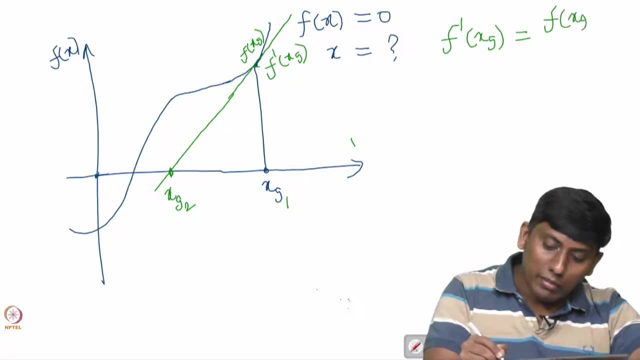 can write. I can write: this is f of x g minus f of ok, So x g 2 divided by x g 1 minus x g 2, right? So this way I can find from this what I know. So this way I can find from this what I know. 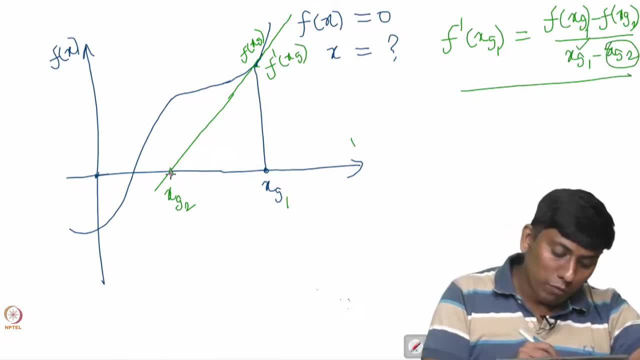 I know x g 1, I want to find out x g 2.. So now, if I actually like see here, So what I can see, this is another slope will come, ok, So you can see. So now, this is actually. 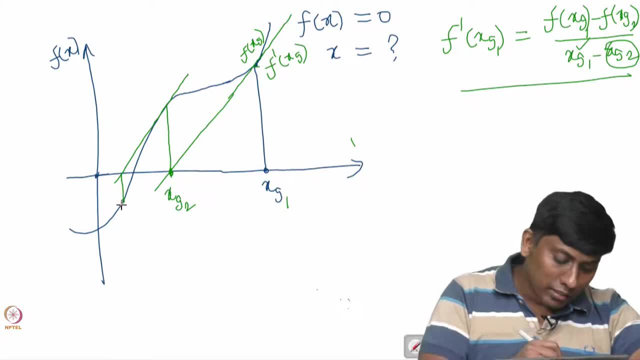 like giving another. you can say iterative point, then I can actually like a make a slope, So then that is giving, So like that. you keep on going. finally, you end up with this point. So this is the basic principle which what you call the Newton Raphson method is. 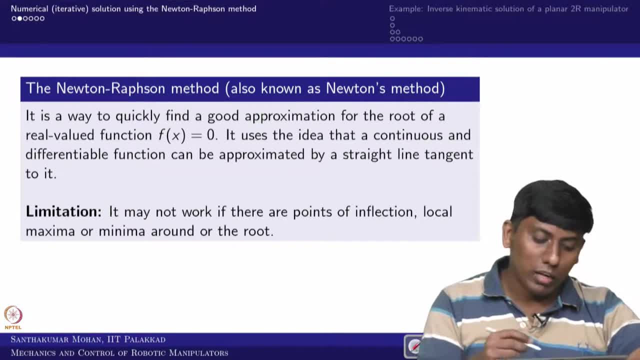 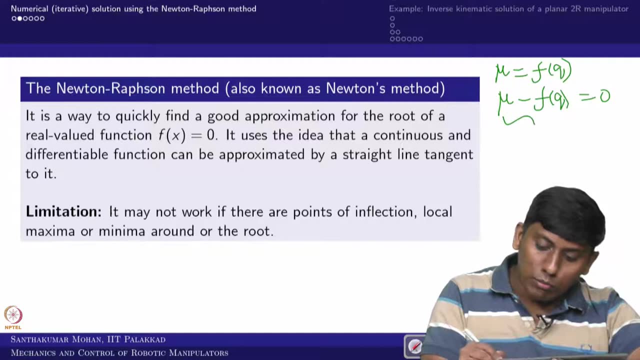 actually like giving. I mean, the limitation is So it may not work. if the, if the, if there are points are of inflection, So what that means. So if it is actually like inflection, So you have something like 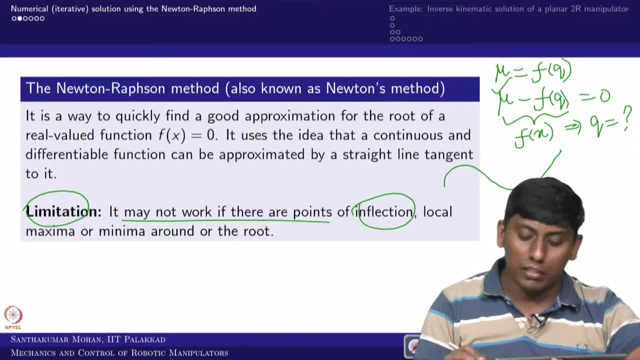 this. you take a point here. this may not actually like reach the another point right. it is actually like come closer here. So now you can see that the original solution- So probably you can see the original solution- is somewhere here. So this is what you can see. this is. 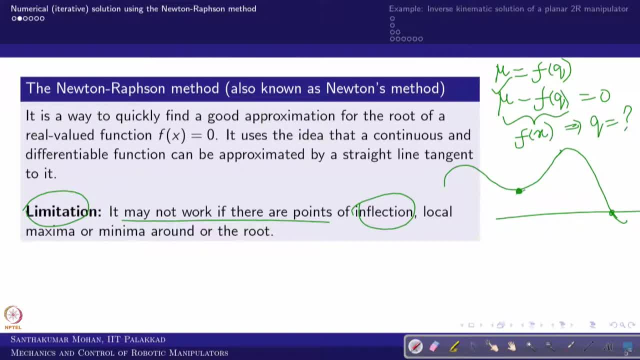 a solution and you have taken a point here. So this point actually like end up with a somewhere actually like close here. that is what we are saying, that the inflection point, but the original solution is here, So which even some people call this, is actually like. 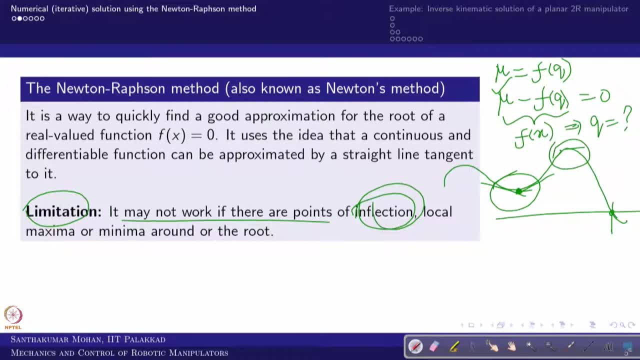 a maxima and this is a minima. this is localized, So if any point is actually like you would chosen your initial guess somewhere here, it would be rotating here itself. So that is actually like one of the limitation in the Newton Raphson method, but still, we can actually. 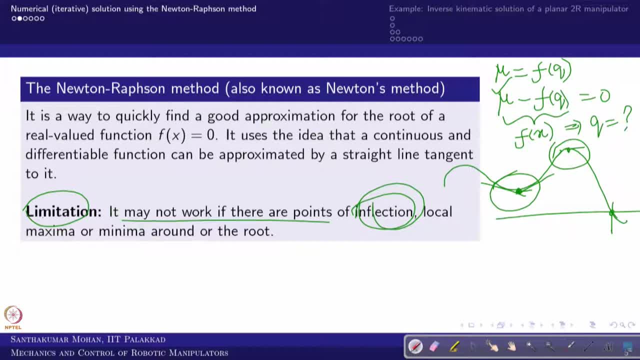 like a try to avoid, by providing something you can say, some additional resistance, So restriction, we can do it. So, if that is the case, So we can see the same Newton Raphson method, what you have actually come across in several, you can say, numerical methods, courses. 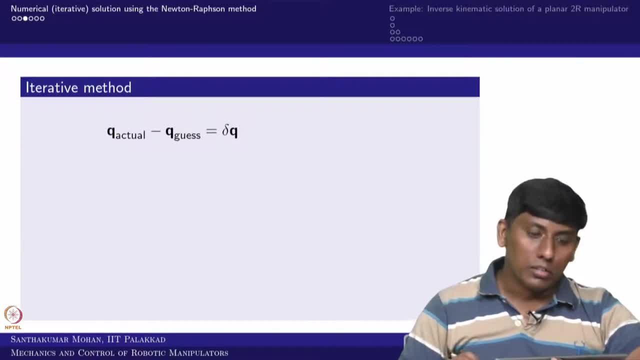 So we are going to modify that in this course. So what we are trying to say that it is iterative method, where we are saying that the actual is somewhere we are actually taking a guess. So the error between these two I am calling actually like delta q, So where q is actually. 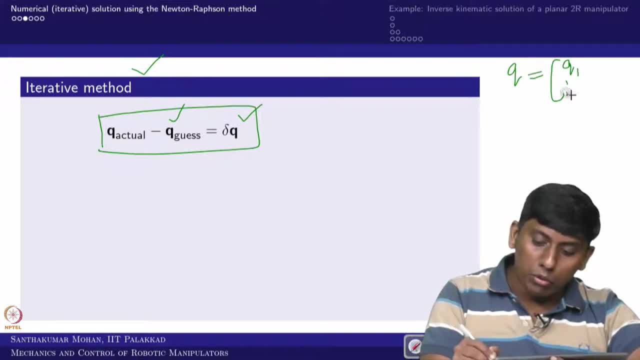 like your joint space. So q1 to qn, this qi can be either so, theta i or di. So if it is actually like a rotary joint, theta i. if it is a translation joint, it would be joint distance. So in that sense, 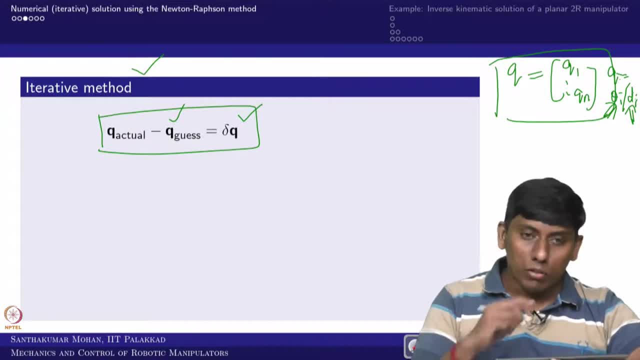 you have a q vector. that q vector would be in this form. So now we are trying to find out the q vector, but we are taking a guess and actual is something. So we do not know the error, but we assume that this is the error. 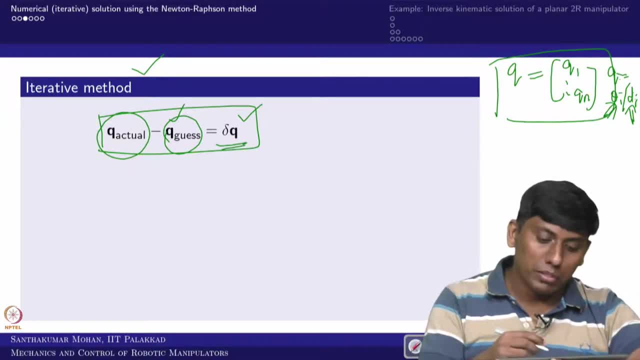 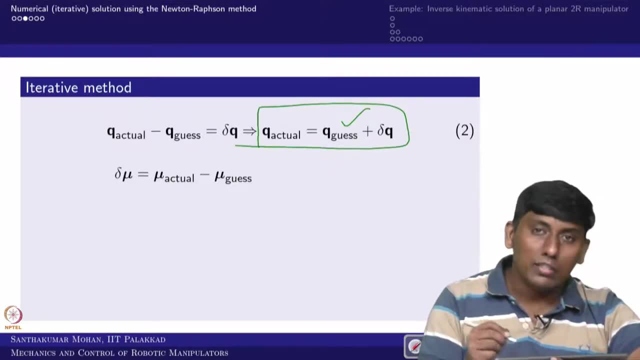 Now, first of all, we would like to rectify or go away from this error for that what we are seeing. So this way, you can actually like rewrite this actual as q guess plus delta q, But what we know, We can actually like a write delta mu, So that delta mu again. 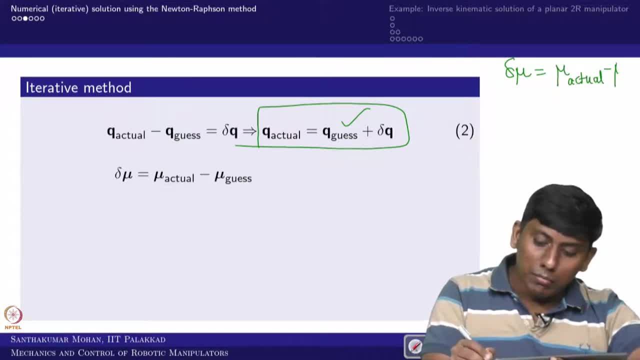 you can write: this is actuaral minus mu guess In the sense. so you know mu is actually like function of q, So you can actually like substitute this guess and then whatever value is coming. that is what mu guess. ok, I keep. 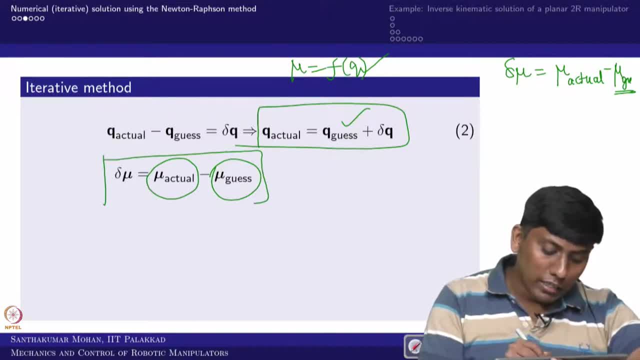 and the mu actual is given. So now what you will get? You will get another error called delta mu. So can we relate anything? Yes, So for that what we are trying to do, So we can actually like take the mu actual, So mu actual what? So it is function of q actual. 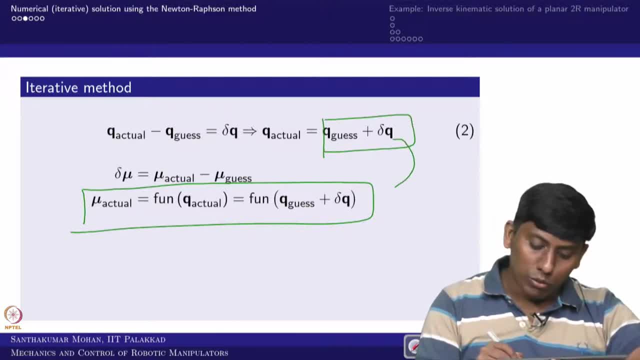 but the q actual is actually like we have written this form right. So now you substitute this, So what you will get: q guess plus delta q. So now you can say mu actual in this form and you use a Taylor series of expansion. So what that will give, So that will give. 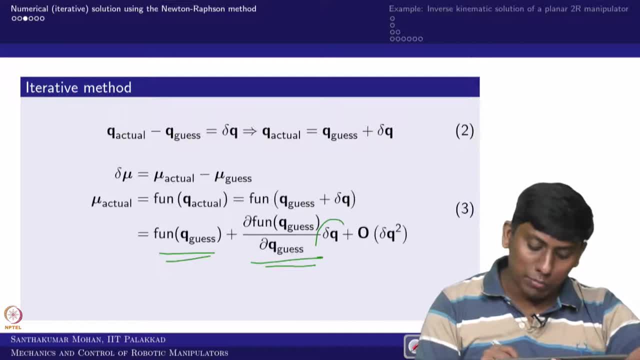 actual like function of q, guess, plus the partial derivative with respect to delta q and the higher order partial derivative multiplied with the delta q squared and other things. okay, So we are actually like assuming that this delta q is very, very small. So this all we. 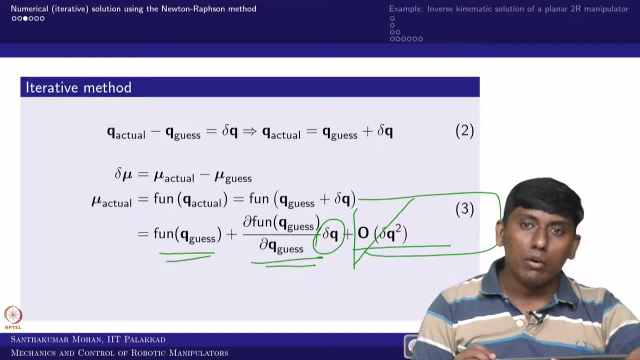 are actually like making it as 0. okay, So now what we can actually see, This is what left, but this is actually like what it is. So you have, f is actually like function of q, So this is also vector and this is also. 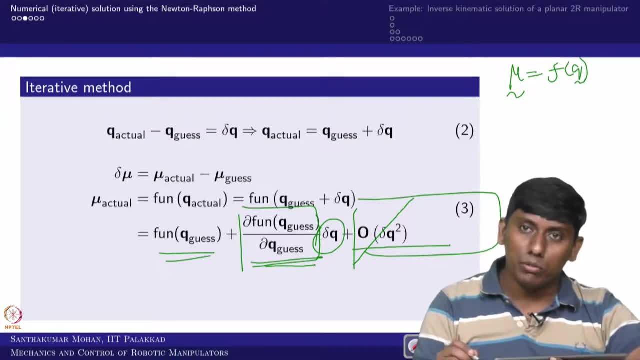 vector. So you are taking a differentiation with respect to- you can say vector differentiation with respect to another vector. So obviously that would be end up with what you call partial derivative. So that partial derivative we are getting. So that is what we are actually. 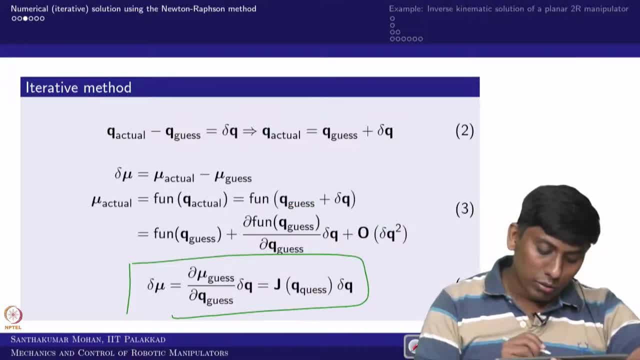 like finding. So, in that sense, what you can write, So you can actually like write, this is your case, So you can actually like substitute mu actual in this form. So this will give mu guess and you have mu actual is mu guess plus this. So if you substitute this, two will go and 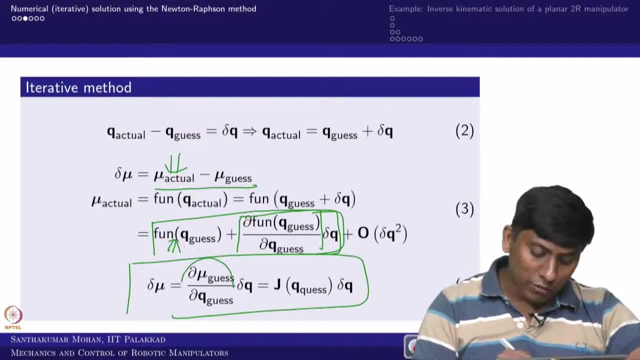 only this would be remain right. So this partial derivative would be in the form of matrix. So that matrix I am calling J of q, guess, which is nothing but a Jacobian matrix. okay, So now, in that sense, what we have actually like end up, We have end up with. 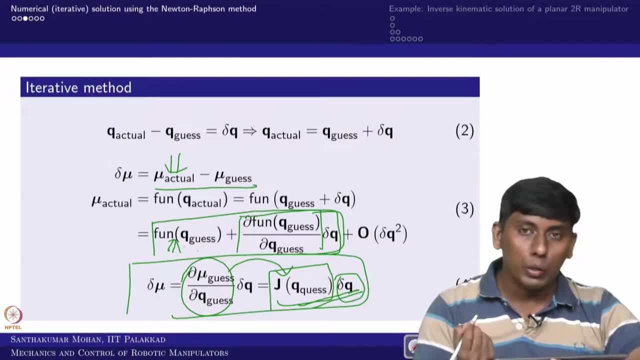 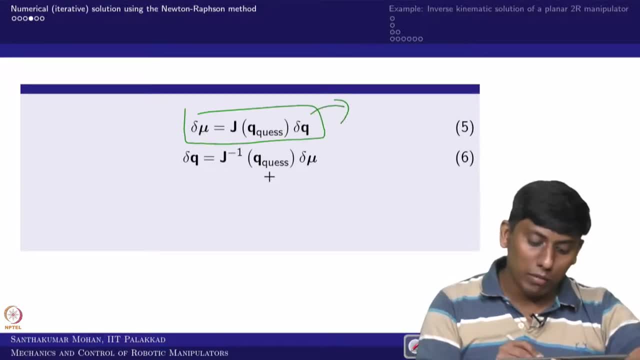 a matrix multiplied with the error. but this error we do not know right. So this is the error we do not know right. So we are actually like rewriting this equation and we are actually like rewriting this delta q in the form of this: So now what? you have this right, So 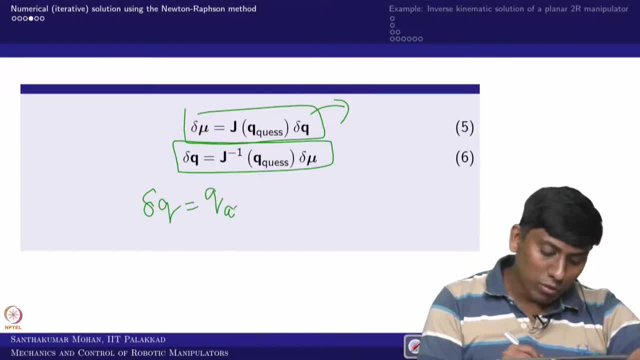 now this delta q is what This is actually like q actual minus q guess, right? So in the sense, what you can do, You can actually like make you actual one side and you put it the q guess the other side. So what you will get, So you will get the final solution. 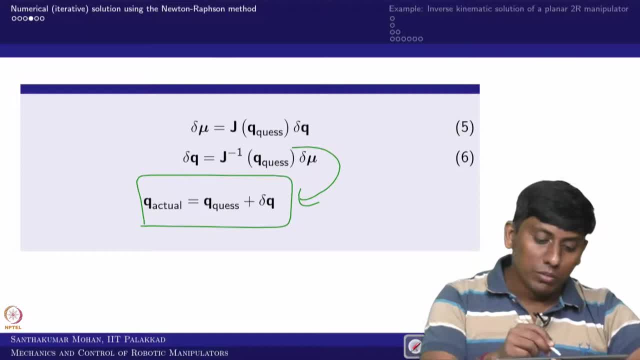 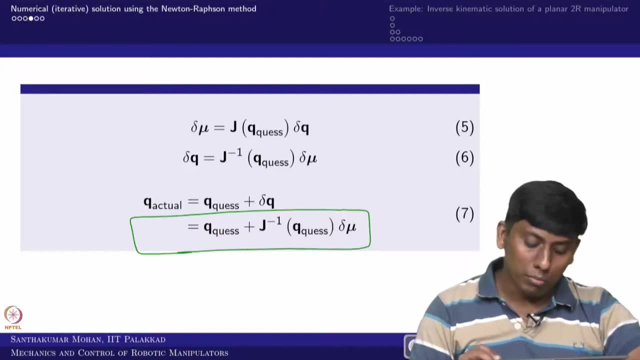 in this form, right? So now you substitute this here. So what you will actually get, This is the final equation which we are going to use in the Newton Raphson method. So now what you can see, So you, once you choose the guess, So you have found this is actually. 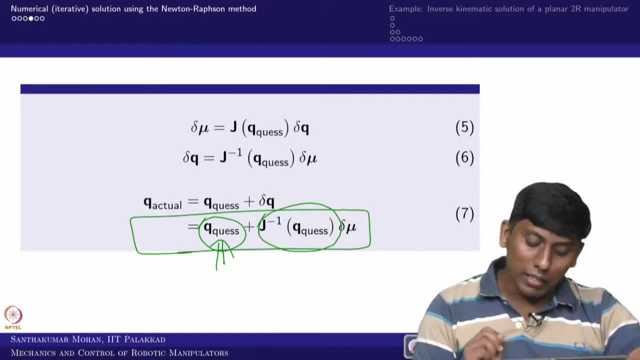 given you can found. you can find k, J and then J inverse you can get. and this is actually like mu actual is given okay, And mu guess you can find because it is function is known to you. So you can actually like get the delta mu and then you can solve the. you can say q actual. 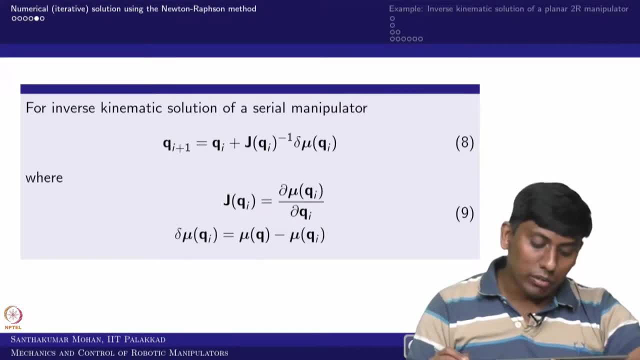 one by one, in the sense iterative. So that is what we are actually like trying to write. So now you can see that the, if the forward kinematic solution is available, we can find the inverse kinematic in a iterative manner, where qi is the initial guess, okay, and J 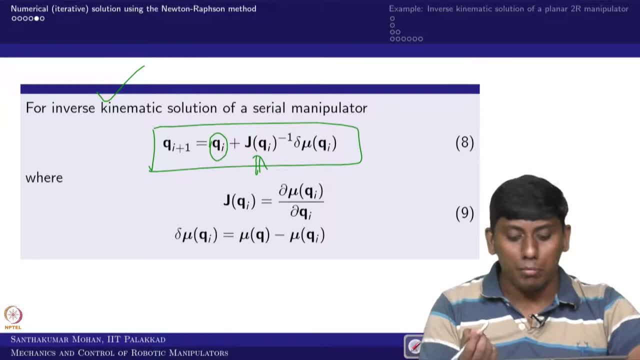 of qi is actually like, based on the initial guess, what is the Jacobian matrix? and this is actually like actual minus your function of. So this delta mu is obtained and once you get, you will get i plus 1. then the next iterative that i plus 1 become i, and i plus 1 would be new value. like that you can actually go. 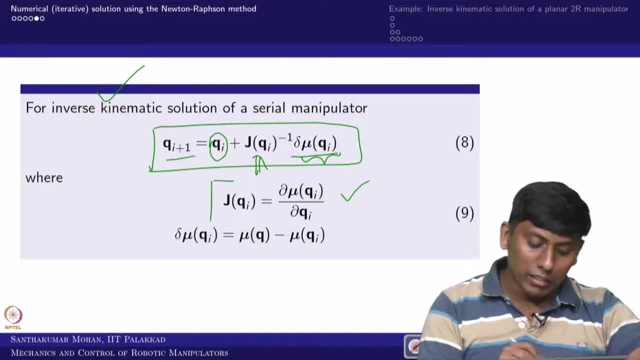 iterative, and that would be obtainable. So here, only condition is: you should have this J. this J is supposed to be non. you can say singular in the sense J of q determinant should be nonzero, Otherwise what happened? this J q inverse would be not possible. okay, So 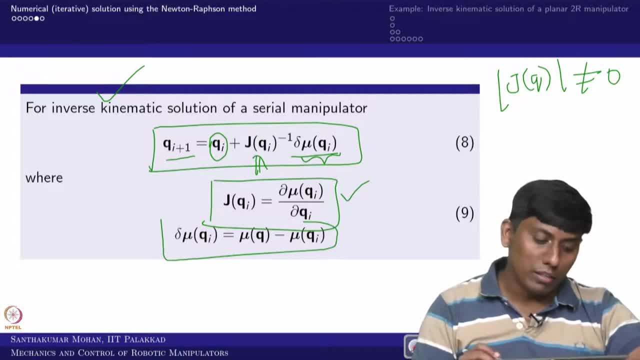 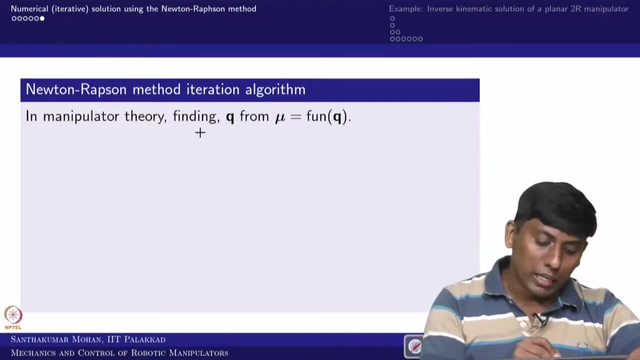 that is what we are actually like writing, So we will take one simple example in the next slide. So for making this as a algorithm, So what we can do, we can actually like start. this is the function. this is available, So we will start with the- you can say iterative. 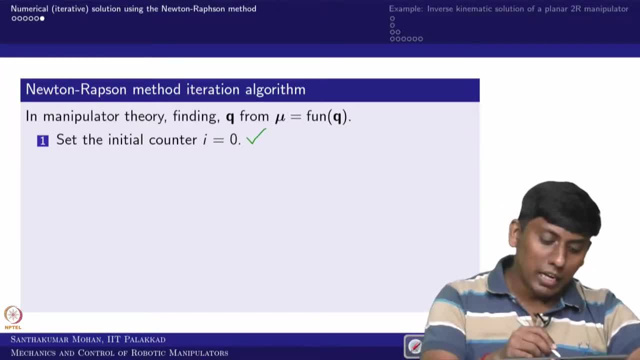 algorithm. So we will start the counter as 0 and we start with the initial guess. So that is what we call actually like qi, that we start. okay, Then we are actually like going with the next step where we calculate Jacobian matrix. 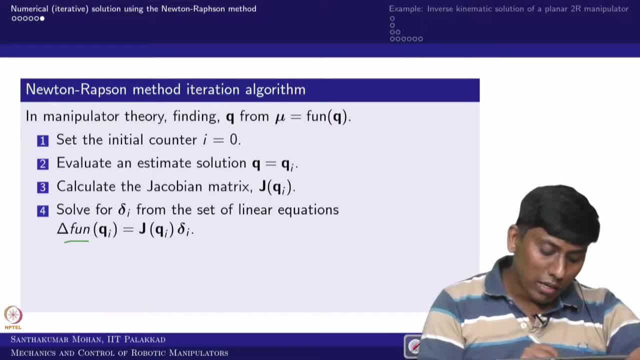 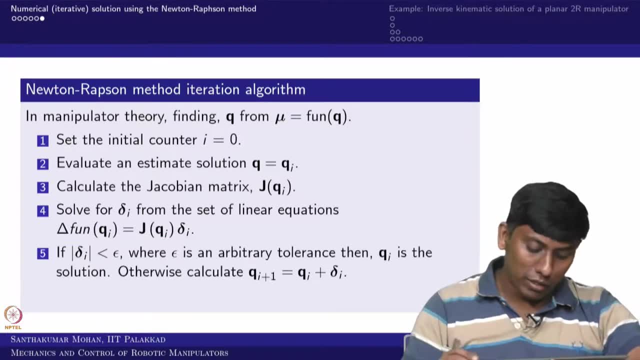 So we will take Jacobian and Jacobian inverse, we calculate and then we will actually like find this okay. So once you actually like find this, then we can actually like keep getting it further and then actually like you can find this particular aspect okay. So in the 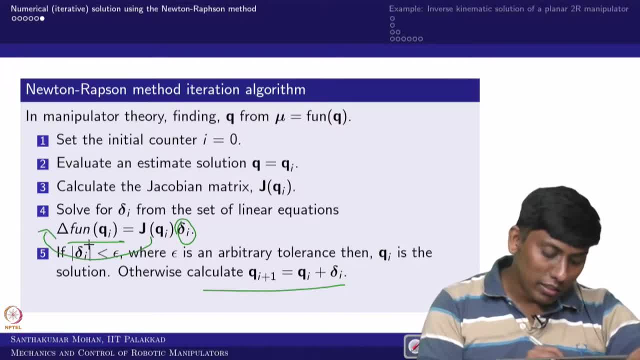 sense this delta i can be taken as this function that you can say the difference in the function inverse actually like obtainable that you can substitute. So in the sense, whatever we have used in the previous slide, that I have really used, So I have actually written this in the form of algorithm. So once you have this, So 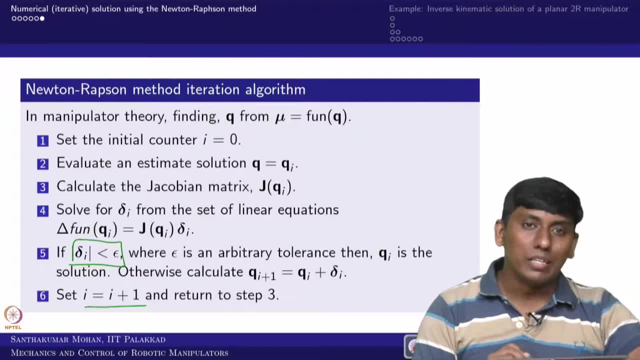 you can actually like stop for stopping. we are actually like putting some. you can say tolerance. So, for example, your delta i is actually like very close to 0, then you can stop. need not to be 0, right? So that is what? so how close So that you need to actually 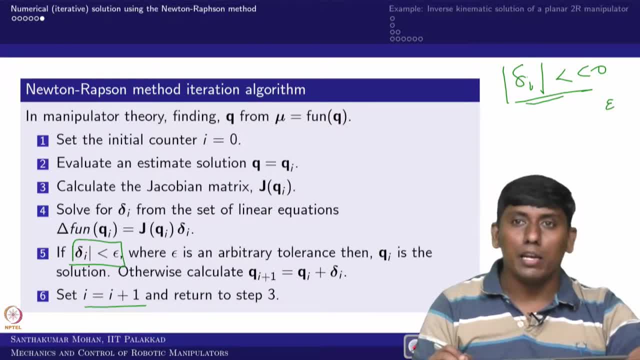 like make your own arrangement. So for that we are taking as a epsilon. So epsilon is your tolerance value, So this epsilon value you can actually like, So with this you can actually stop. So this actually like choose. based on that, you can actually like restrict this algorithm. 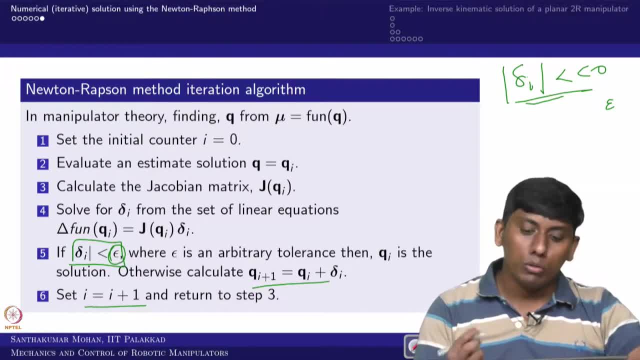 For example, you are actually like running in online, So you no need to go the epsilon as 10 power minus 10 and all You can even restrict, 10 power minus 1 is sufficient. you can stop it. So that is the criteria here. 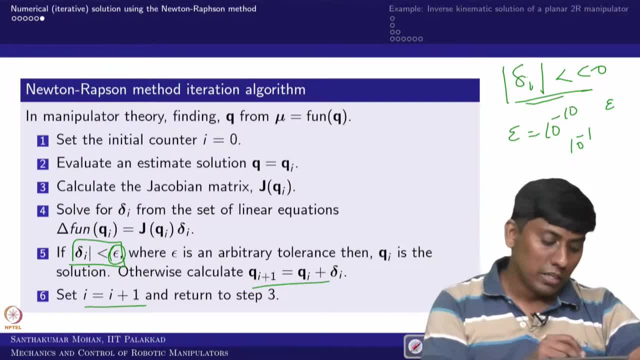 So now you can see the same thing, what we have written in the equation form. that is written in the form of what you call algorithm, The same algorithm. we will try it in a numerical example, So then you will get much more clarity how this algorithm work. 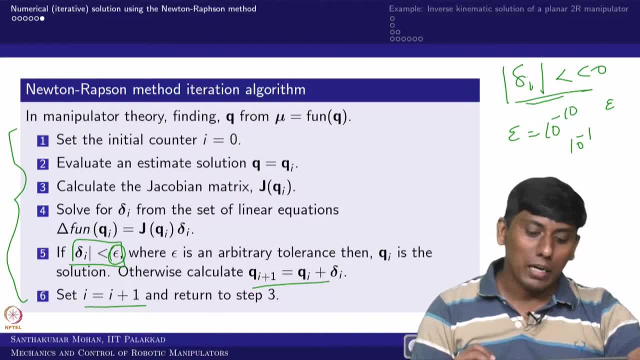 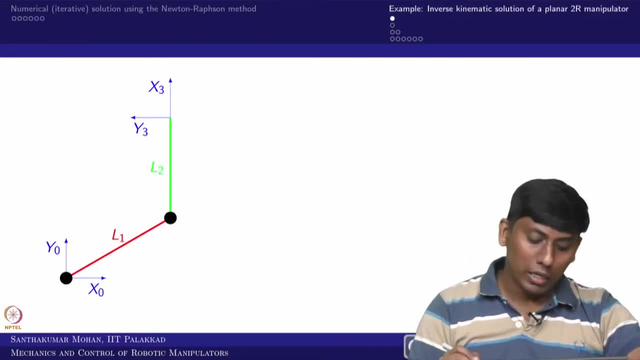 In fact the next lecture, I would be showing this in the MATLAB simulation, or you can say MATLAB algorithm base. So we will see. So now let us actually like move the numerical example. For that we are taking a 2R serial manipulator. 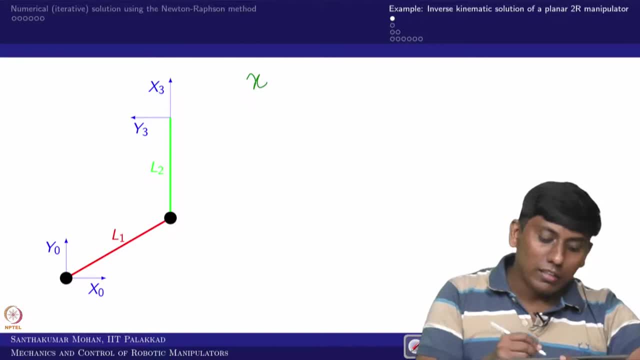 So we know, like this, right. So what would be the x position of this? this is actually like x and y, So this x would be L1 cos theta 1 plus L2 cos theta 2.. So theta 1 is actually like this angle and theta 2 is this angle. 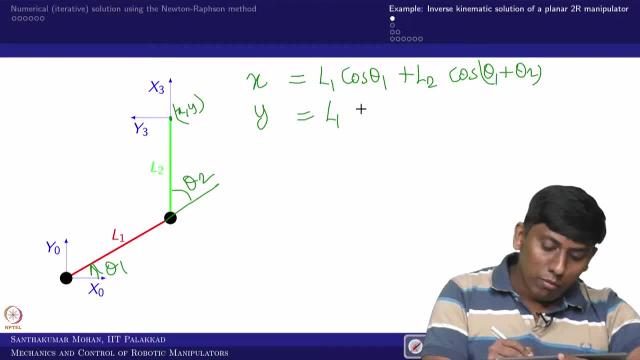 So we can actually get this So similarly. y is so L1 sin theta 1 plus L2 sin, so theta 1 plus theta 2.. So now what we are saying. so if we know these two, can I find theta 1 and theta 2 numerically? 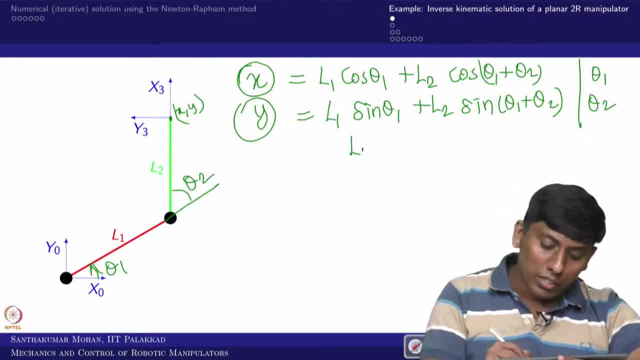 Yes, So for that, what are the things supposed to be known? Yes, So theta 1 should be known and L2 should be known. These are geometrical parameter right which are supposed to be given. So, in addition to that, what actually it would be given to you? 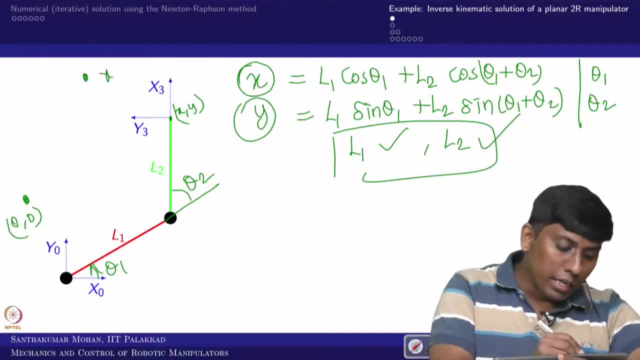 So it would be like 0, 0 and your x, y would be given and L1 value would be given, L2 value would be given. So you are actually like trying to fix this in the form so that you can find theta 1 and. 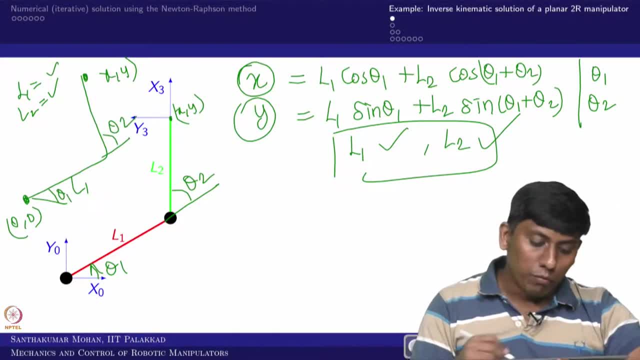 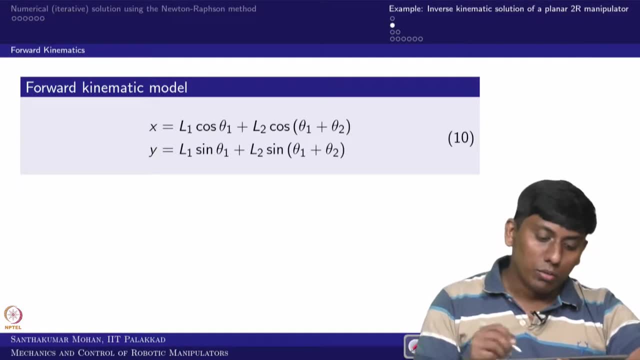 theta 2, right, So this is what we are trying to do. So for that, what one can do, We can actually like go The forward kinematic model. So this is what I have written. So now you can take the partial derivative. what that means. 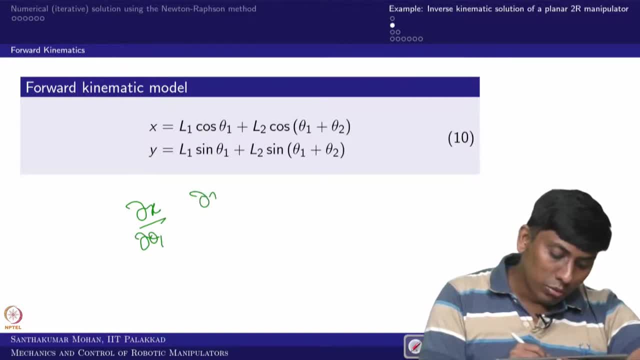 So dou x by dou theta 1, okay. So dou x by dou theta 2 and dou y by dou theta 1 and dou y by so dou theta 2, right. So this is actually like what you call Jacobian matrix. 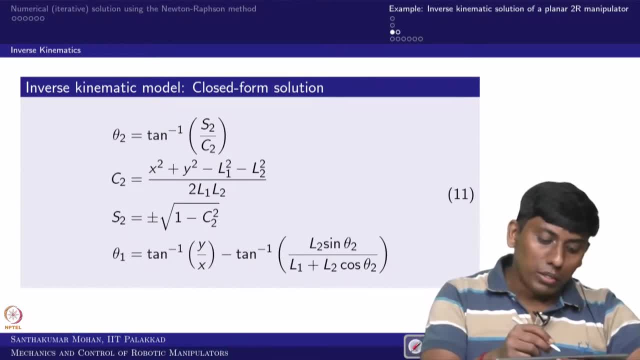 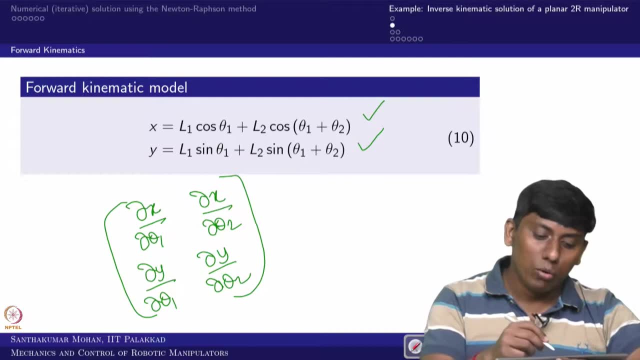 So you can actually like find So before that, what one can see. So this is actually like forward kinematic. So this is actually like forward kinematic solution is known and we have already the closed form solution, which are already available. So that is what this. just for comparison, I am taking this. 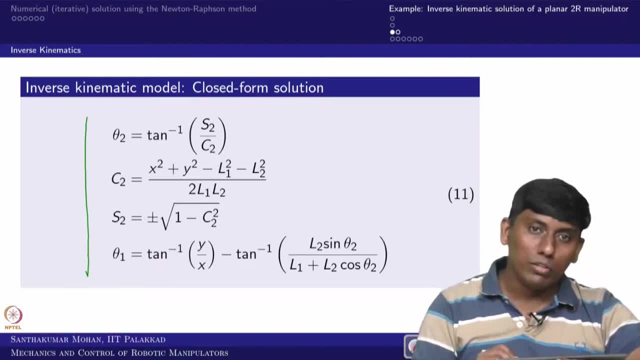 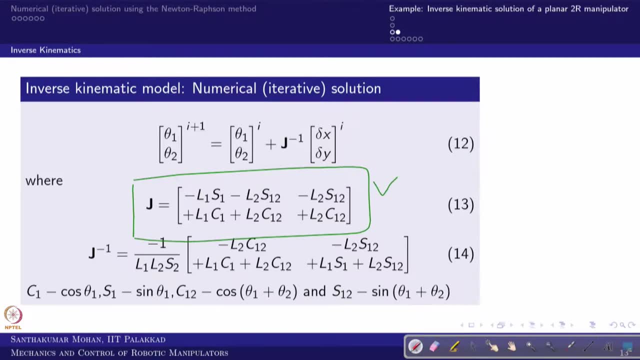 So this is we have already solved in the last class, So the same solution. I have put it here. So now you can see like what we need to know, this Jacobian matrix. So this is we have obtained and this is the algorithm which is actually like we have formed. 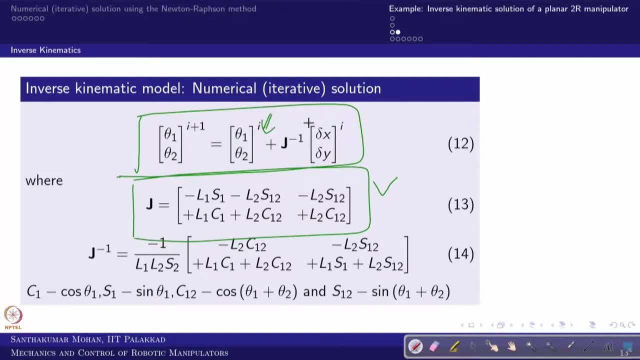 So now we are actually like starting with the initial guess and based on the initial guess. So we find the Jacobian inverse and this delta x and delta y, then we can go again, right? So then you can see we are taking one of the numerical example. 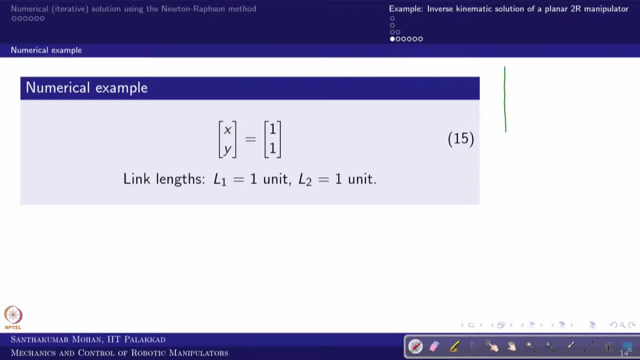 So where x and y is 1 and 1 in the sense you take, this is actually like your x axis and y axis, and this is 0: 0.. So what you have obtained, So this is so 1 comma 1, okay. 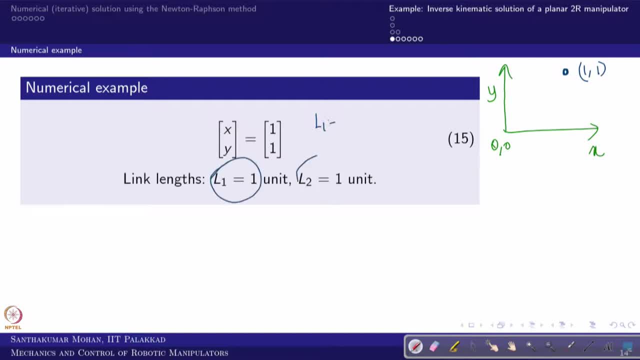 In addition to that, what L 1 is actually like 1 unit and L 2 also 1 unit. So what you have obtained. So this is so 1 comma 1, okay. In addition to that, what L 1 is actually like 1 unit and L 2 also 1 unit. 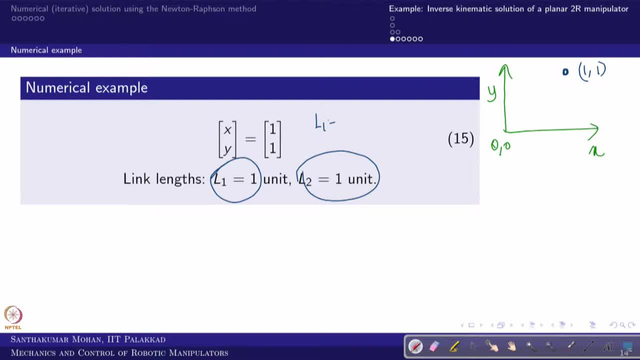 So, in that sense, what is the best possible solution? So you can easily see, the possible solution is: so this is 1 unit and this is 1 unit, right? So L 1 and L 2, you can fix it, or what you can do. so you can fix it this way, right? 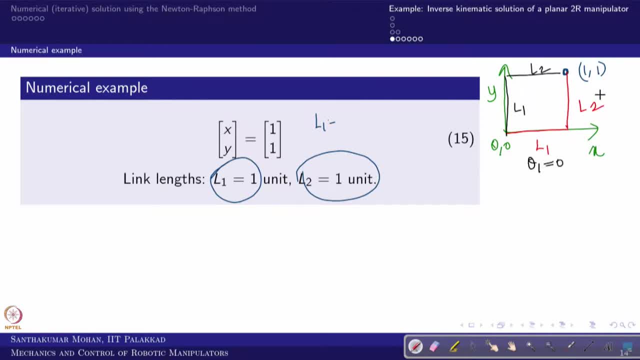 So in that sense theta 1 is 0 and theta 2 is actually like 90 degree is one solution. The other solution is: so: theta 1 is 90 degree and theta 2 is minus 90 degree. So this is one solution. 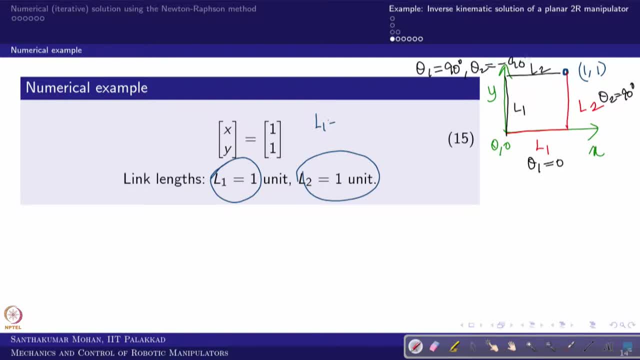 So this is one solution. So theta 2 is minus 90 degree is second solution. okay, So these are the two solutions which we have actually like obtained. So in that sense, so you can see, like can we actually like find the same solution in numerical? 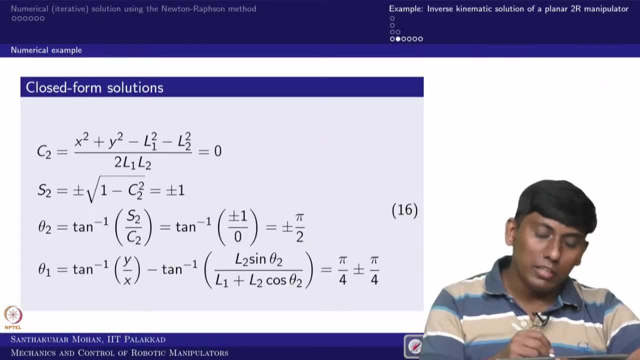 example. So for that first, we are actually like substituting this into the closed form solution which we know. So you substitute L 1 and L 2, and x and y, all are 1.. So in the sense, this would give 0.. 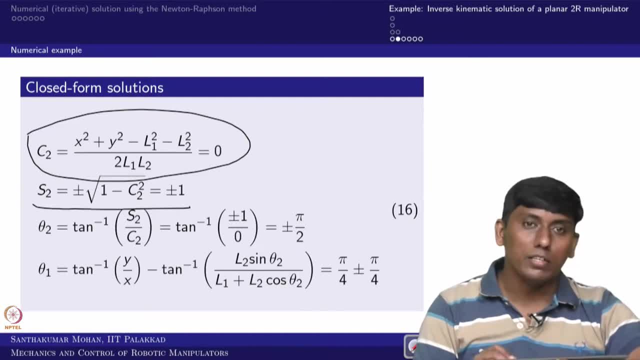 So what is S 2?? S 2 is actually like plus or minus square root of 1.. S 2 is actually like plus or minus square root of 1 minus C, 2 square. So that would give plus or minus 1.. 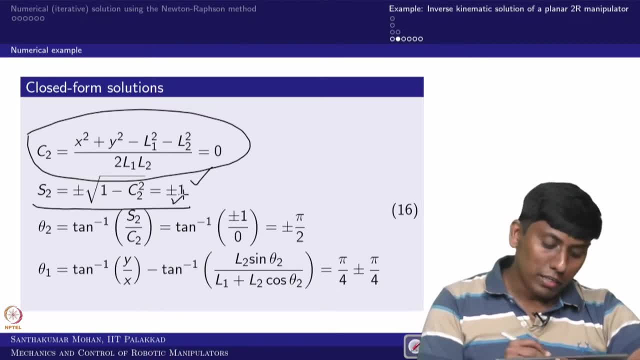 If you take plus 1, that would give one solution. If you take minus 1, that will give another solution. If you take plus 1, what happened? this is 1 by 0. So in the sense, this is actually like infinity. So this will give pi by 2, okay, right. 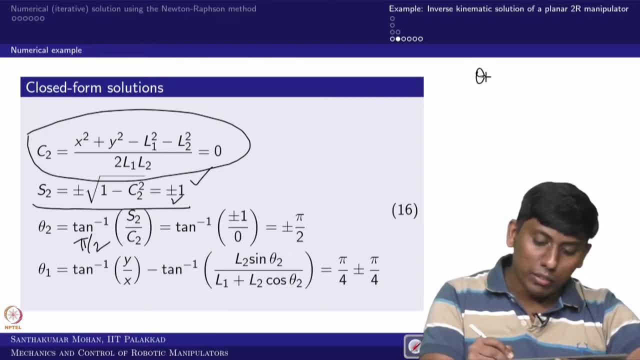 So, but it is actually like if you take plus 1, so theta 2 would be, so pi by 2, so then theta 1 would be So tan inverse of 1, this is pi by 4, and this is actually like what happened: this become. 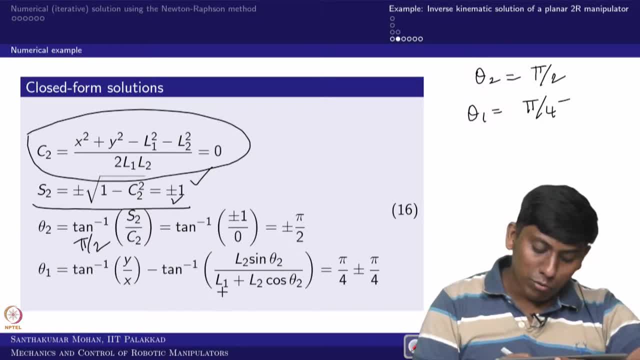 you can say 90. So L 2 would be there and here L 1 would be there and this would 0. So in the sense, what we will get, 1 by 1.. So in the sense, minus pi by 4, right. 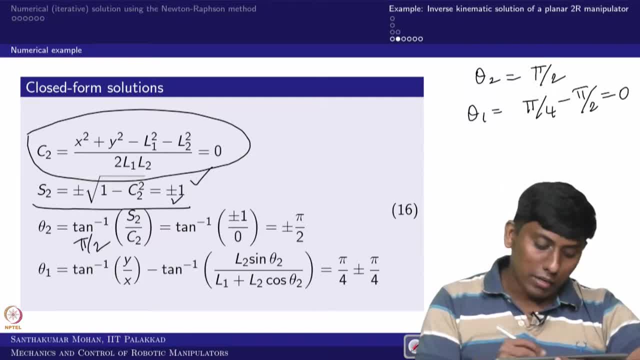 The same, theta 1 is 0, right, If you take it is actually like minus 1. so then theta 2 would be minus pi by 2.. If you take this, this is minus 1.. So in the sense it is actually like minus pi by 4.. 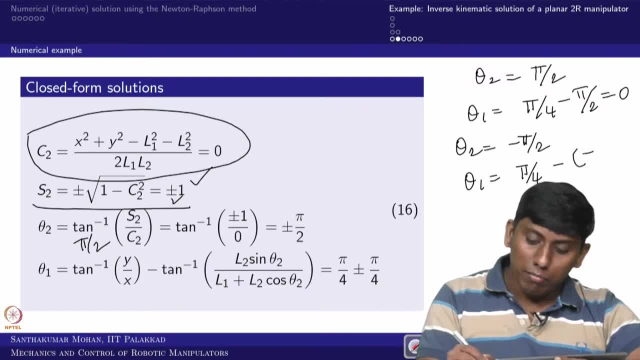 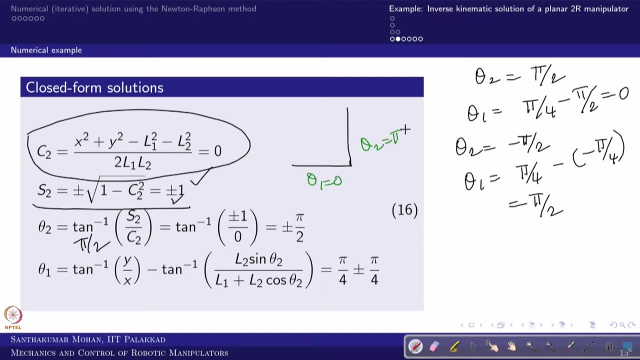 This and theta 1 is so pi by 4, minus of minus pi by 4.. So in the sense, it is actually giving so pi by 2, okay, So the same solution, what we have obtained, this is one solution, okay. So in the sense, theta 1 is 0 and theta 2 is actually like pi by 2.. 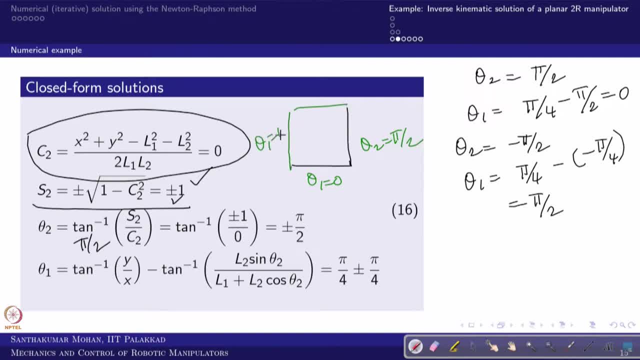 So the other solution is this: So theta 1 is pi by 2 and theta 2 is minus pi by 2, right. So both the solution we have obtained. So now, So you can actually like see the same thing- can be obtainable in the numerical basis. 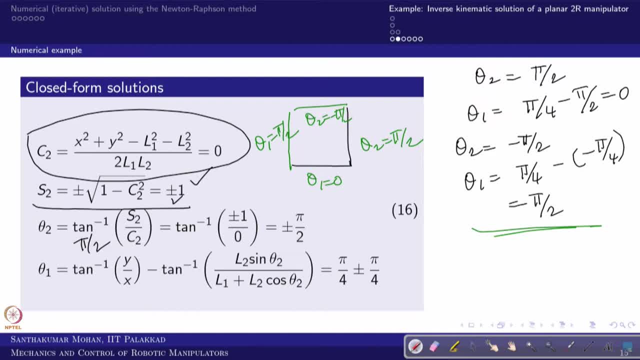 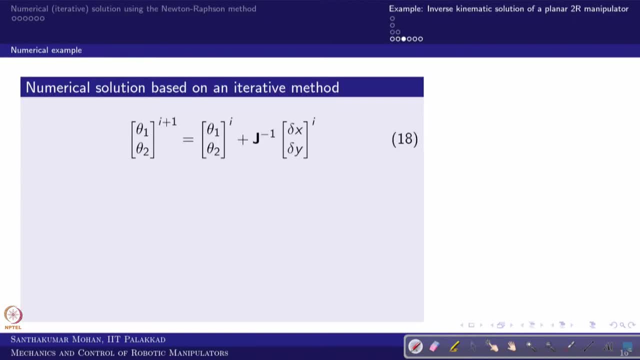 So what that means, So you can actually like try to apply the algorithm which we have done, So that we are actually like trying to see: okay, So these are the two solutions. So we are actually like taking into this case, So now what you can see. so you are taking an initial guess. 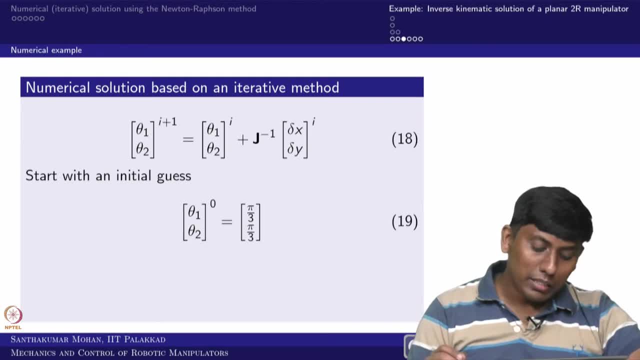 So initial guess can be anything right. So what can be initial guess? So initial guess: I am taking a 60 degree each. So if I substitute this, So what I will get? So I will get delta x something, because so 1 and 1 is given and this is the mu actual. 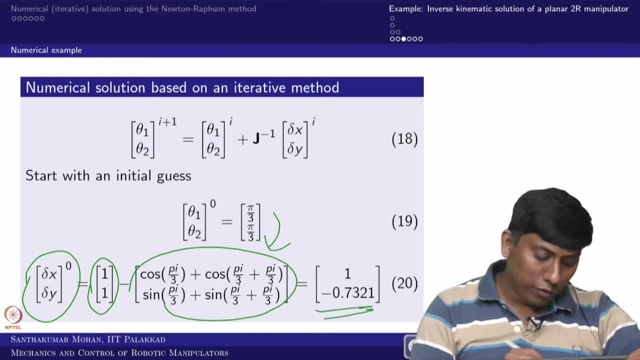 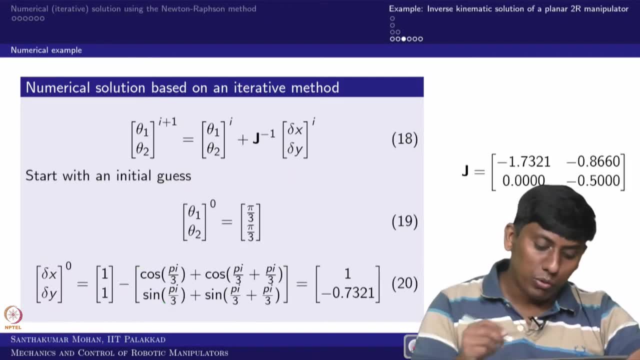 based on this initial guess. okay, So now this is the difference in the delta mu. This is equal to delta mu. This is the value and J inverse I need to find. So I substitute that value into. you can say here: So the J value is obtained. 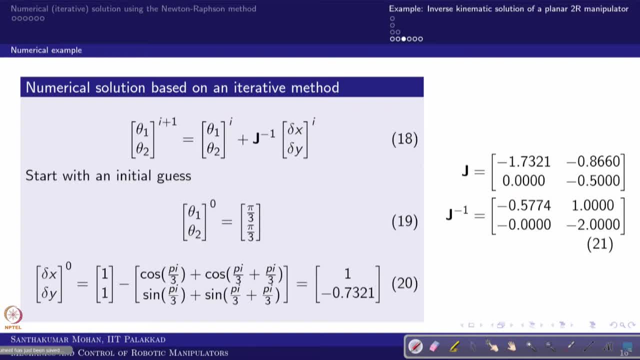 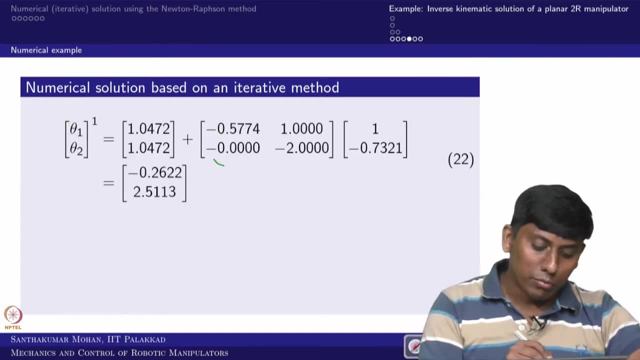 So then I can do J inverse, right? So then what I can do? So Then J inverse are there, So I can go again with the algorithm. So I can actually like substitute the J inverse and the delta mu is obtained. Initial guess is there. 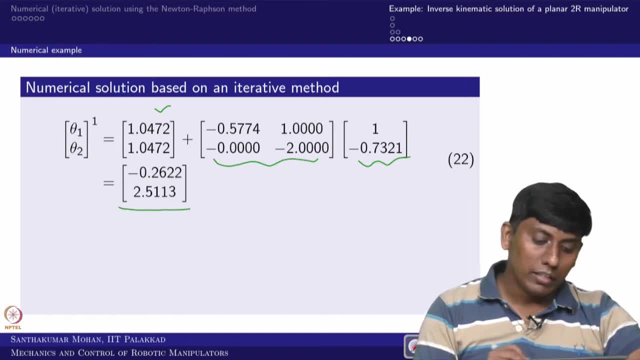 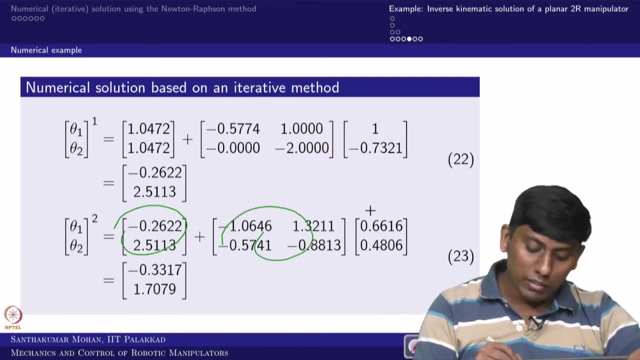 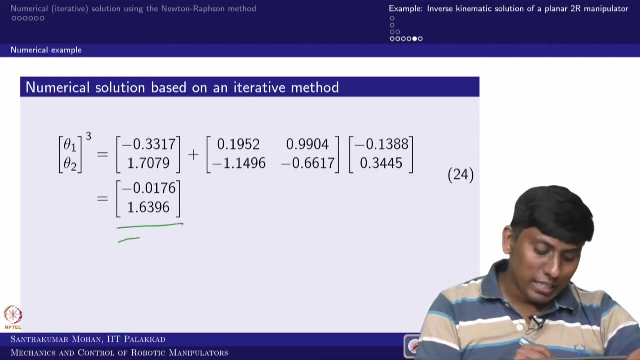 So I will get nu. you can say qi, right. So now, based on this again, I will actually like calculate delta. you can say mu, the J inverse, this is delta, mu and the initial guess, and then I will get So like that if I keep on actually like going it. so what you can see, it is actually like 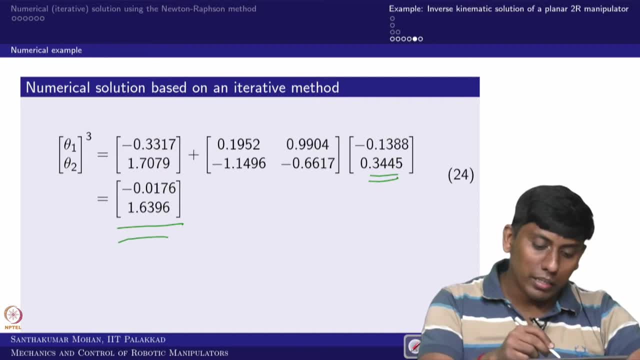 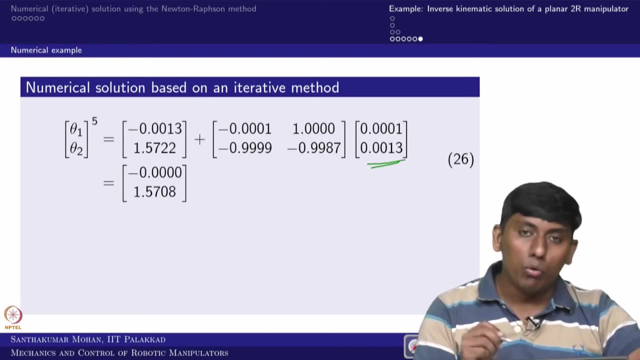 coming closer and closer. Okay, So you can see, right, This value is actually like getting closer and closer, in the sense getting reduced, and you can see one point of time it is actually like coming. So 1 e power minus 3 ratio and you, even you can see, this is coming. 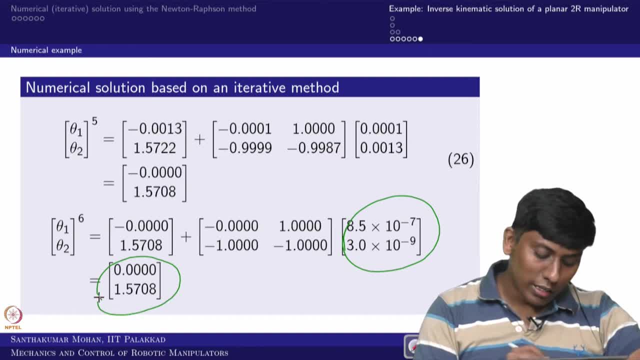 So 10 power minus n in the order. So now you can see this is actually like equal. So this is 0 and pi by 2, right, So pi by 2 in radians, if you write it, is 1.57, something, right. 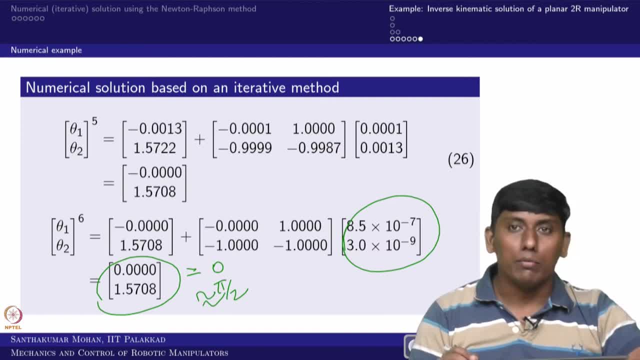 So in the sense, this is equal. So now we have actually, like, obtained whatever we have actually obtained. Okay, This is actually like a derivative. So now, if you are taking instead of the initial guess is actually like 60 degree and 60 degree. 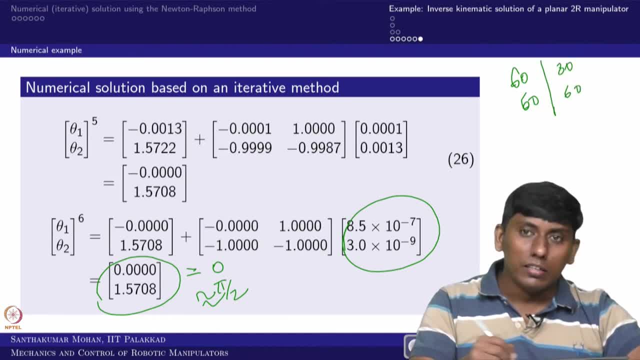 If you are actually taking probably something like 30 and 60, the iterative may be taking time. If you are actually taking 30 and minus 60, it may be it may be ended with the next solution. What is the other solution? 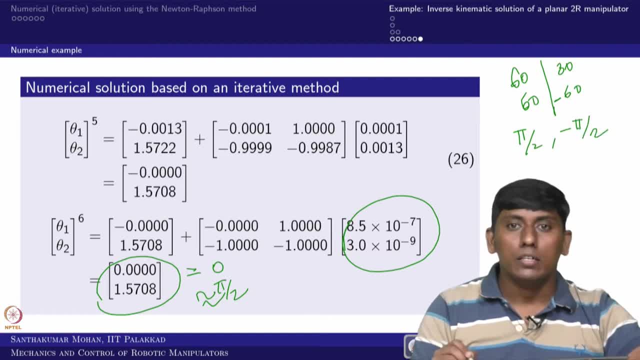 It would be actually like pi by 2 and minus pi by 2.. Okay, So only one condition I am putting here. so whenever you are substituting, you substitute in the common unit. So you substitute in the radians. okay, Because your Jacobian matrix would be, in the order, different and you are actually giving. 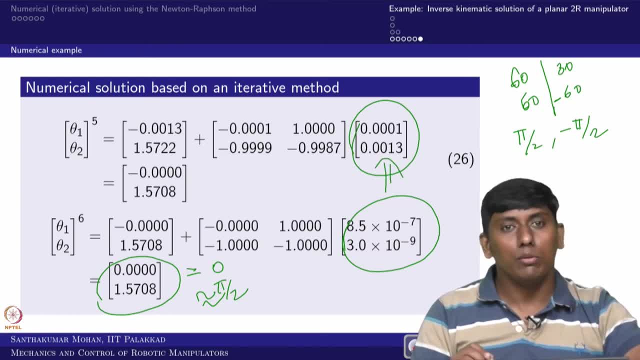 your position, values actually like in meter, better you use in radians everywhere. So now these values are in radians So you can convert that into degrees whenever you require. So with that we are actually like end up with Newton Raphson method. So now the same method can be applied to any serial or parallel manipulator. 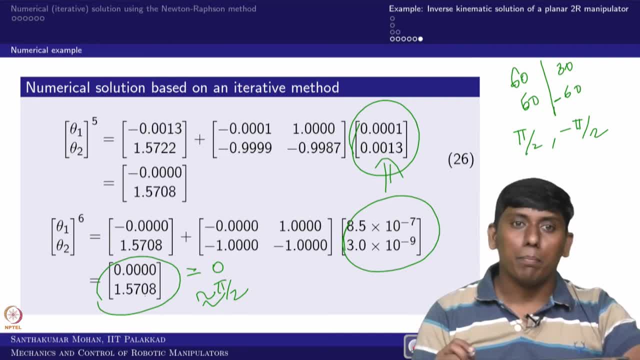 But this course is actually like restricted to serial, So you can actually like apply for the serial manipulator. So even you can actually like go for 6 DOF system or 3 DOF system. It can be RPR or RRR or RPP- whatever manipulator you have, you can actually like apply.